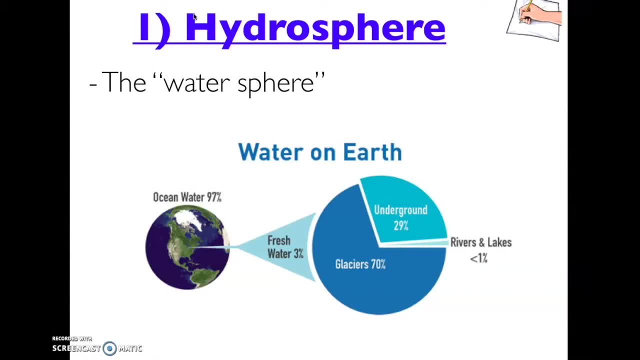 However, of that 3%, 70% is locked in glaciers and ice caps, meaning we don't have access to this fresh water. And then 29% of that fresh water is groundwater found deep within the earth, and we would have to pump it in order to access it. 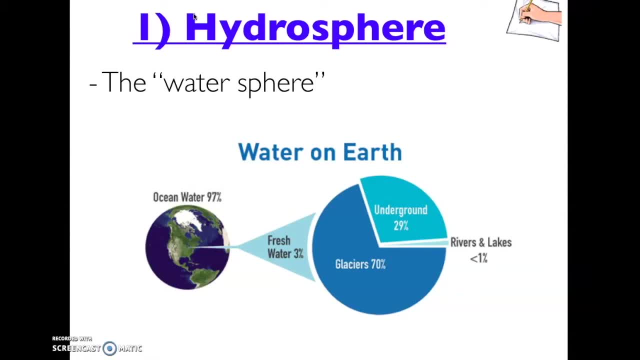 This leaves us with less than 1% of the 3% of fresh water for available use. Water is very precious. Although there is much of it on our planet, there is a limited amount that we can use, which is why we should be careful to conserve it and to use it properly and efficiently. 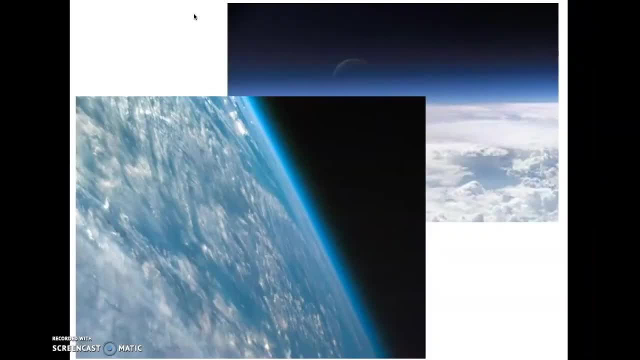 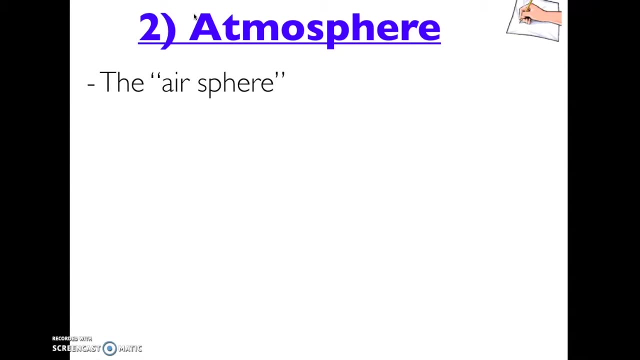 The next sphere we will discuss pertain to these images. Number two: atmosphere. The atmosphere is the air sphere, because atmos means air. The atmosphere is what helps to maintain earth's temperature. It protects organisms like us from the sun's ultraviolet or UV radiation that can be harmful if we are exposed to too much. 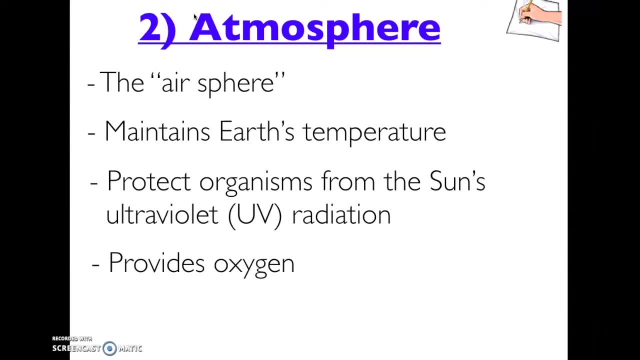 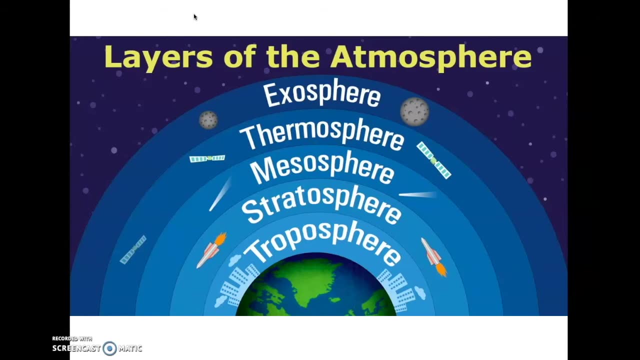 The atmosphere also provides us with necessary elements and gases like oxygen that we breathe in, such as oxygen and oxygen. Not many people know that our atmosphere is made up of five layers. They are the troposphere, stratosphere, mesosphere, thermosphere and exosphere. 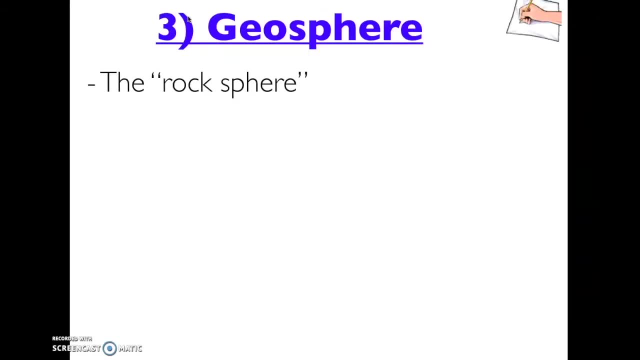 The next system is the geosphere, also known as the rocksphere. The geosphere includes earth's layers, which are the crust, mantle and core, and how they form. It also includes rocks and minerals that we find on earth- fossil fuels. 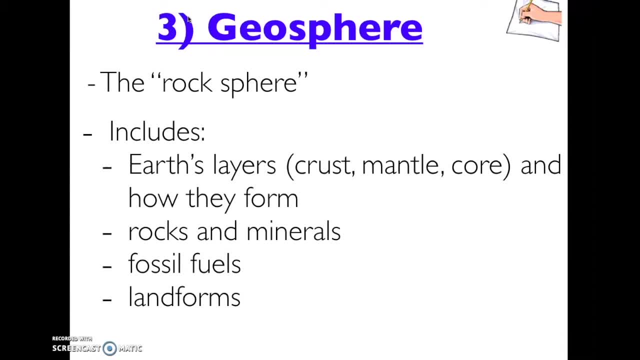 which include coal, natural gas and gasoline, which we find within the earth, having been formed through fossils, and also different land forms of earth. You may have heard of geology, which is the study of earth, including all these topics: The percentage of earth's water to land. 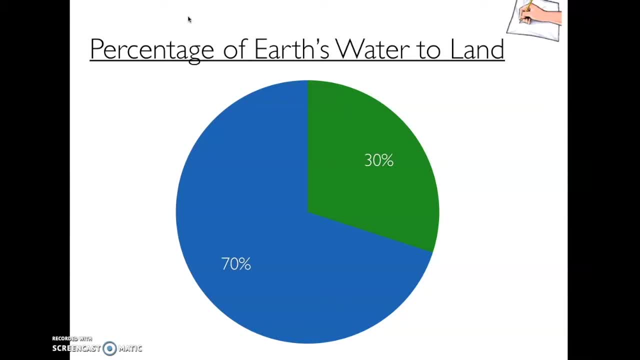 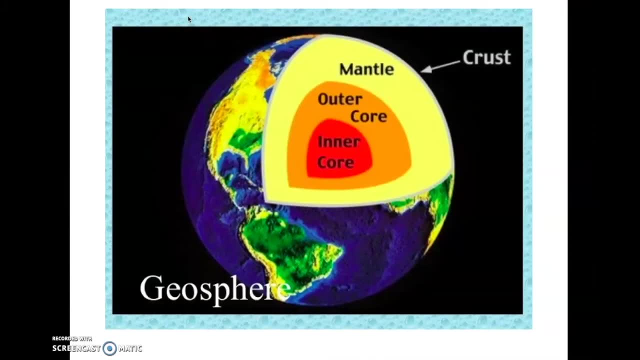 Seventy percent of earth is made up of water, so the blue represents water and 30% of earth is land. next we see a diagram that shows us the different layers of the geosphere. the outer layer is called the crust, which is the layer that we 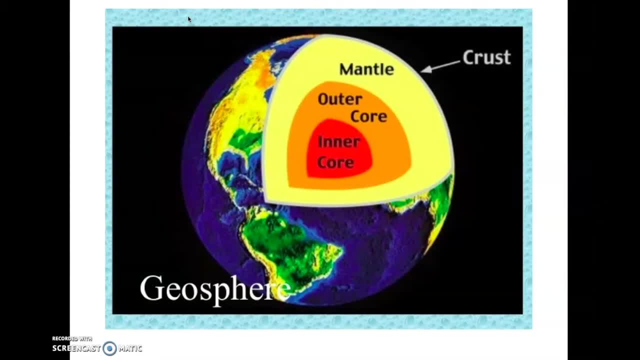 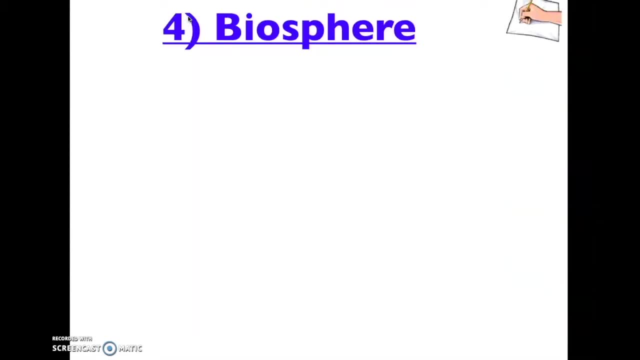 live on. underneath it is the mantle, and underneath the mantle are the two layers of the core, the outer core and the inner core. finally, number four, biosphere. the biosphere is the life sphere. it includes all living things and we see here, listed all the kingdoms. we have different animals. 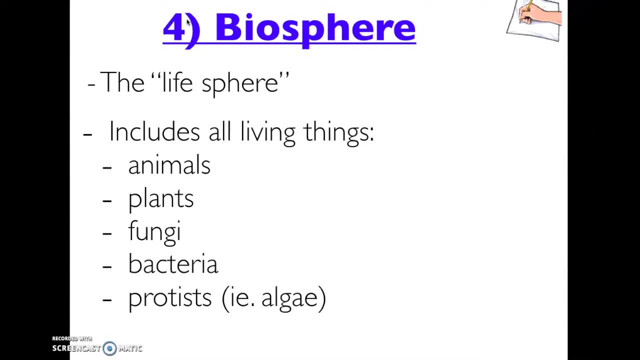 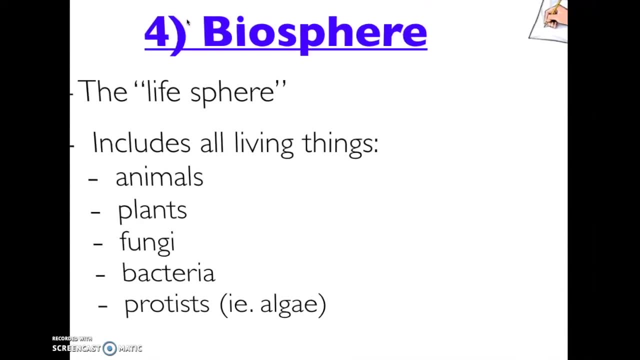 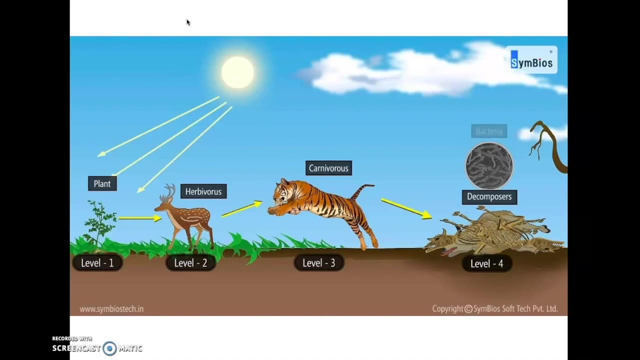 like us, plants, fungi, bacteria, which includes you bacteria, and arca bacteria and protists such as algae. and here's an image of an energy diagram. we see the plant as a producer, receiving energy from the Sun, giving energy next to the herbivore, which is the deer. 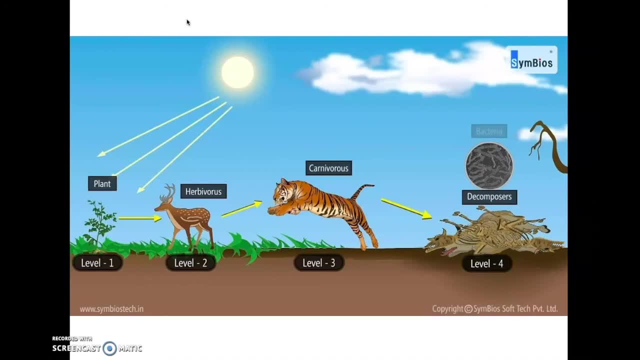 who gives energy to the tiger, who is a carnivore, and the secondary consumer, but it doesn't end. their energy then gets transferred to decomposers like bacteria that break down dead and decaying materials and return it back into the earth so that the whole cycle of life can begin again. but 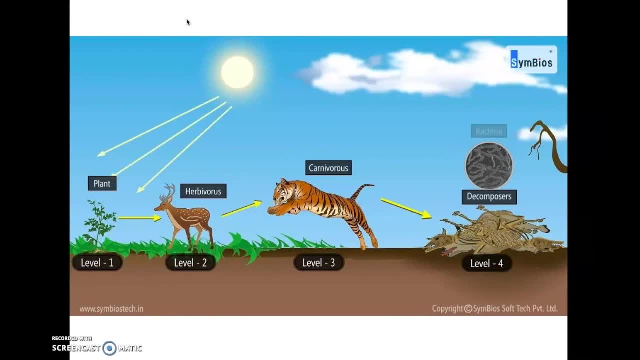 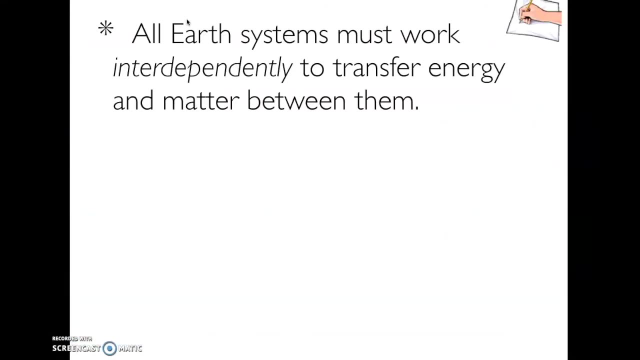 as a reminder, the initial source of energy is the soil, and the soil is the soil and the soil is the, the sun, and this is what we call a food chain. In summary, all earth systems must work interdependently to transfer energy and matter between them. The word interdependently means that they have to 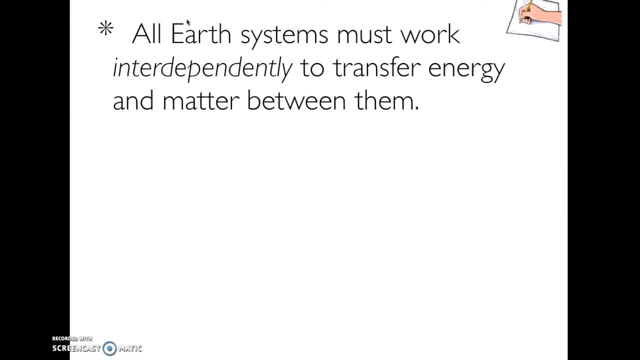 depend on each other. So the hydrosphere and the geosphere, and the biosphere and the atmosphere, all must function together, transferring energy and matter between them for the whole earth to function. Here is an image of four spheres interacting together. We see our air sphere. 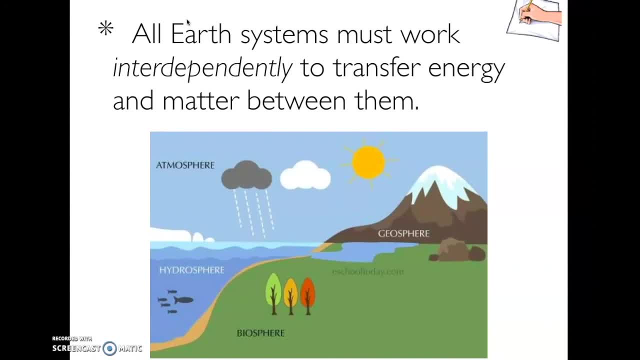 the atmosphere, as well as the ocean, which is our hydrosphere. We also see the biosphere in the fish and the trees and the grass, and we see the geosphere, which are the different landforms, which has the mountain in the background.